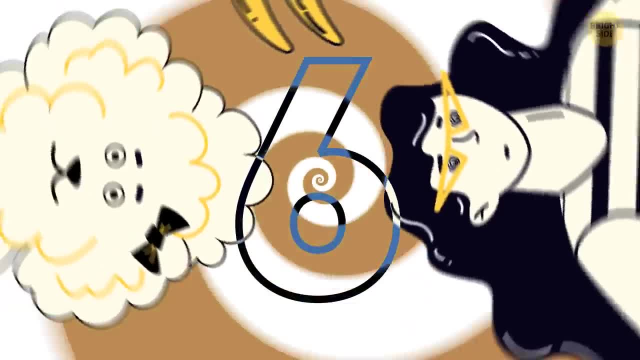 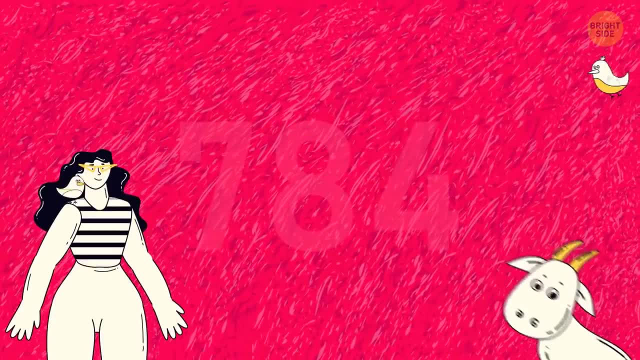 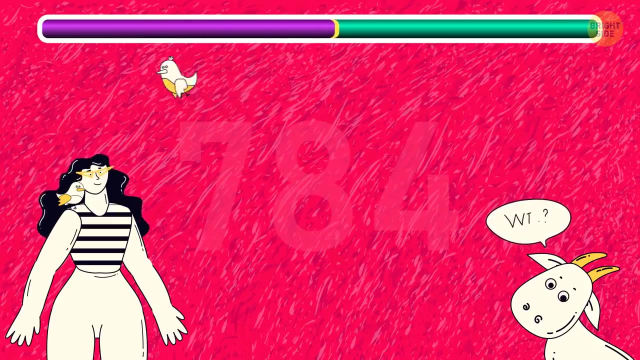 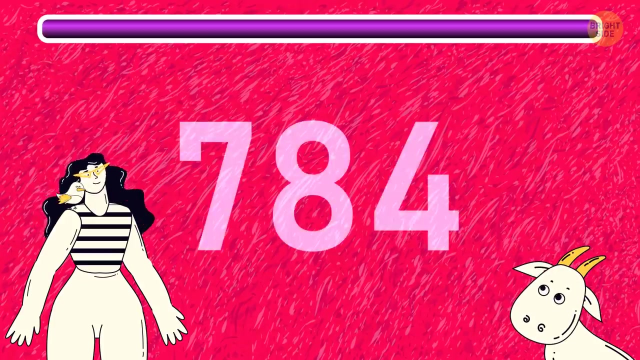 You'll have 10 seconds for each of the optical illusions. Your task will be to read the hidden number. You'll go from the easiest to the hardest riddles. Start off with an easy one for warm-up. Told you it's 7.84.. 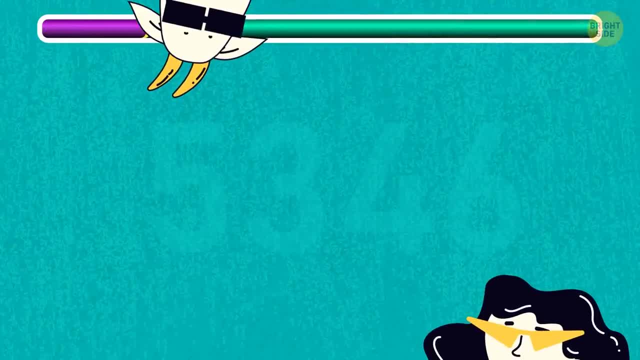 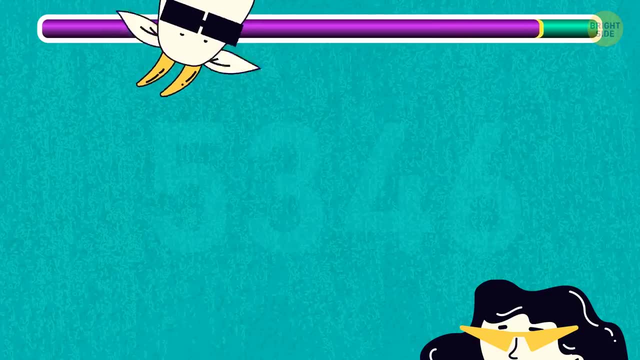 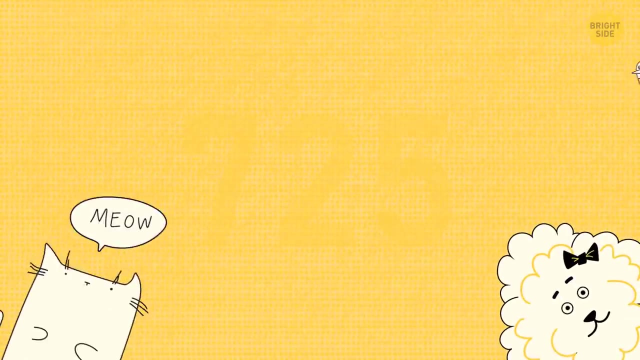 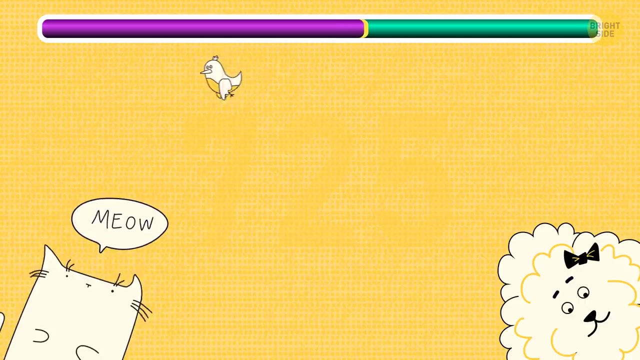 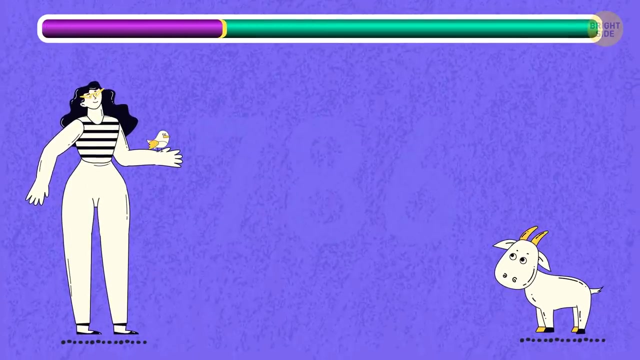 Moving on. I hope you were able to see the number 5346 here. Level up. How about this one? The correct answer is 725.. And another one: Yes, it's 786.. Now, only 5% of people can read the next three numbers. 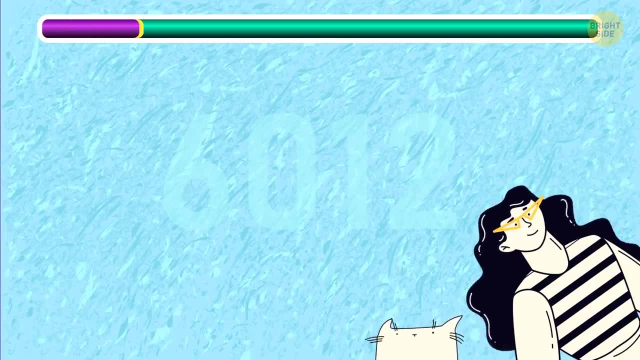 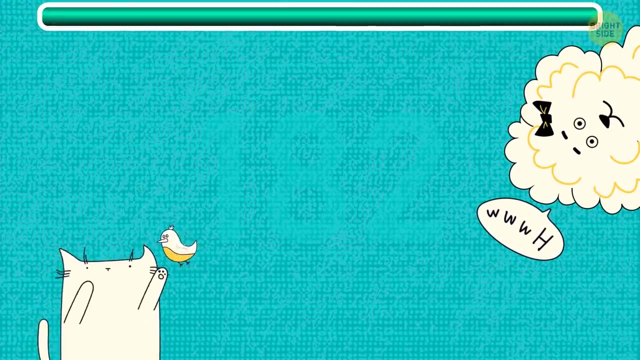 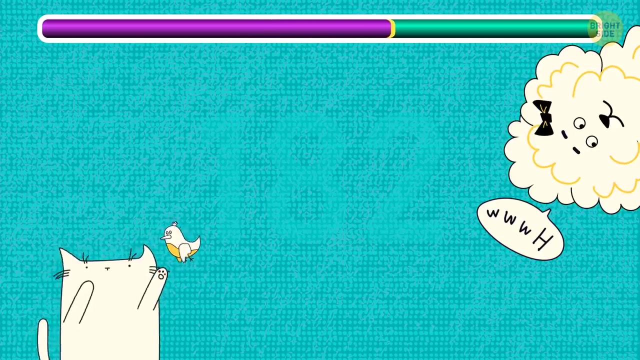 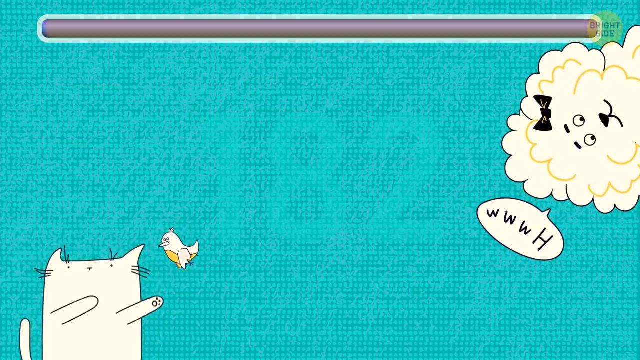 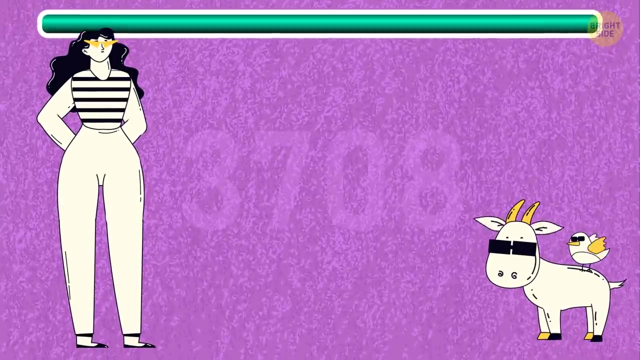 Want to give it a go. If your answer is 6012, it's correct. And here's another tricky one: It's 182.. And if you saw it, you must have eagle vision Told you it won't be easy, but try this one. 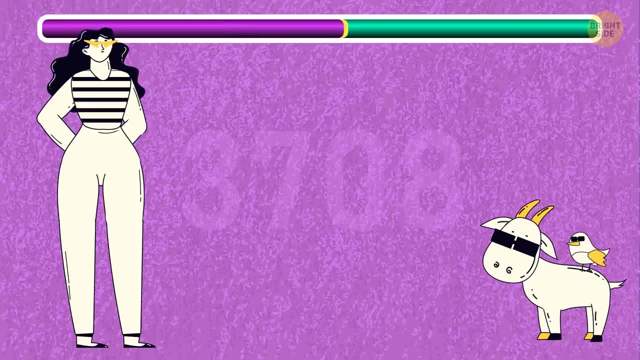 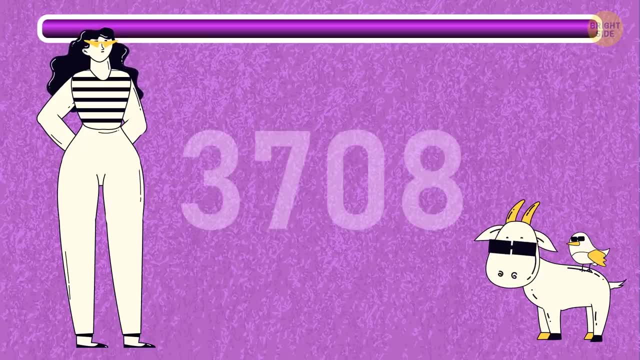 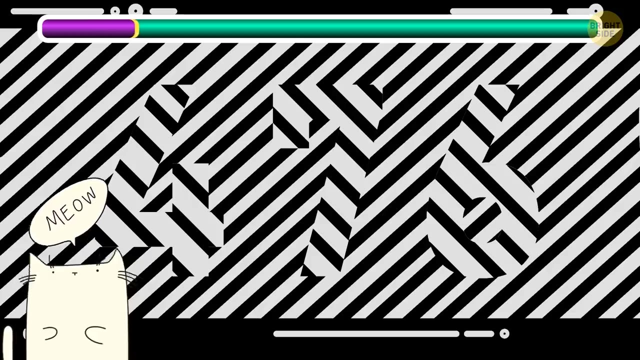 Ask your child if they can read 60&10.. I wish I knew 60&10.. The correct answer is 3708.. Can you see it? It can read 0.. Now, 20 times How, how It can hear. 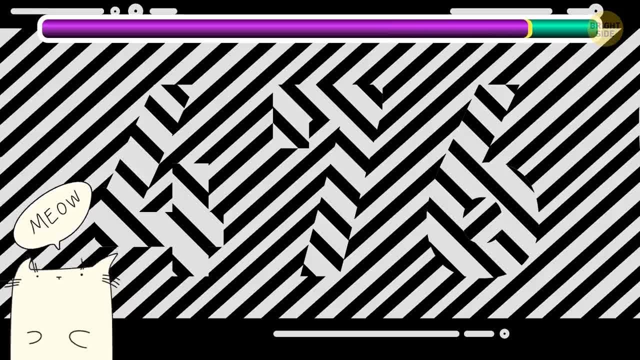 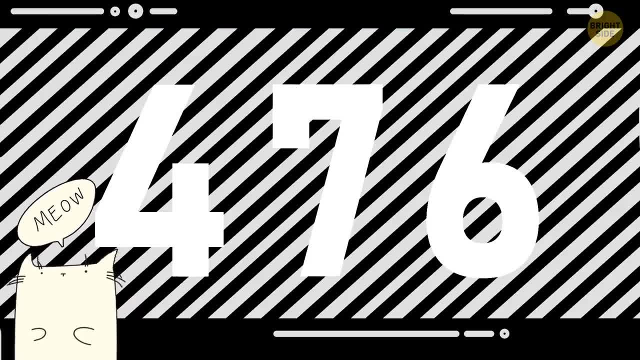 10 seconds away from touchdown. How could that be? It can read 4200.. Even 10 times past demotivation, overwhelming. And the first one is hiding the number 476.. There you go. If that was too simple, how about this one? 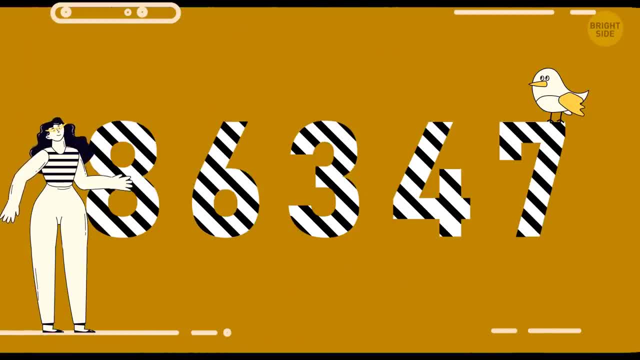 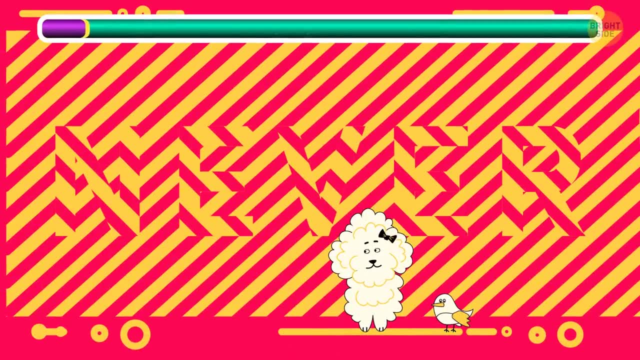 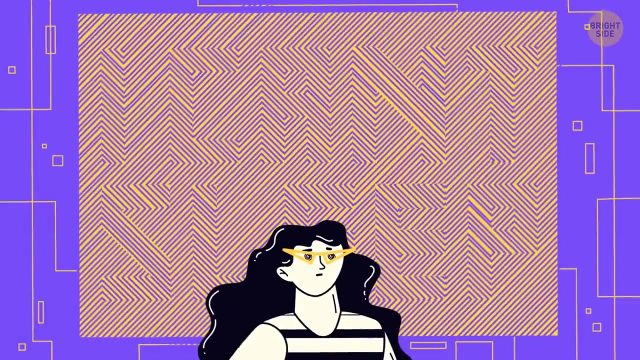 I hope you guessed it was 86347.. And now let's test your eyes with some hidden words. You still have 10 seconds for each of them. I'm sure you figured out. It's the word never Can you read what this picture says? 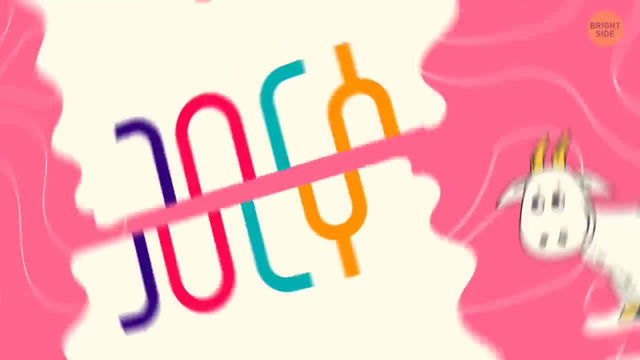 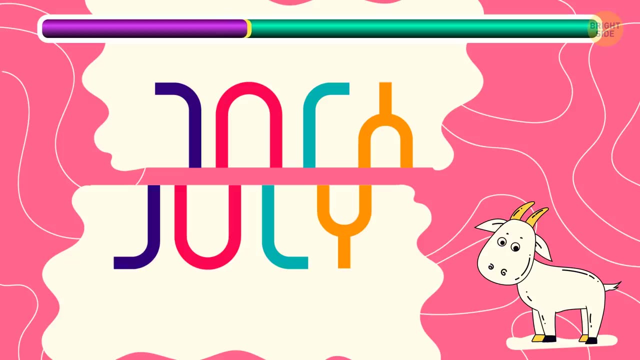 I can't sleep. How sad This one is hiding the name of some month. You have to think outside the box to read it. Feel free to pause the video if you need more time. Well, the secret was to split it in half. 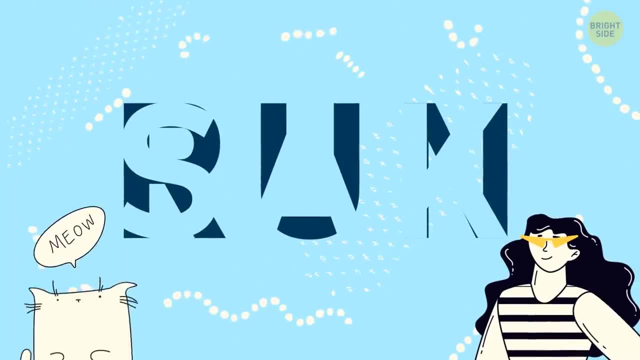 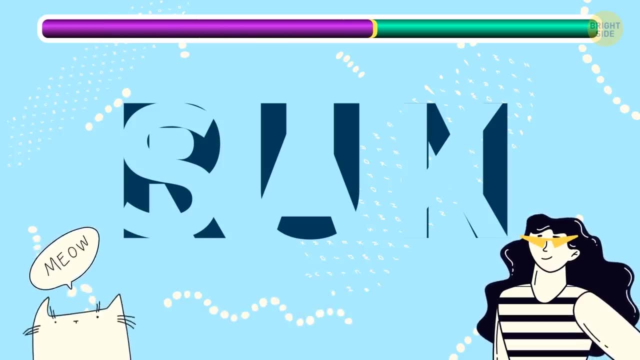 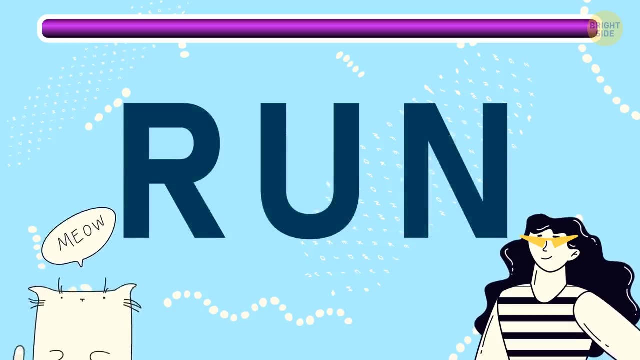 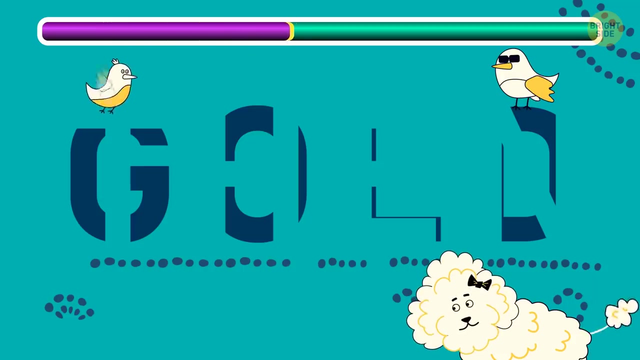 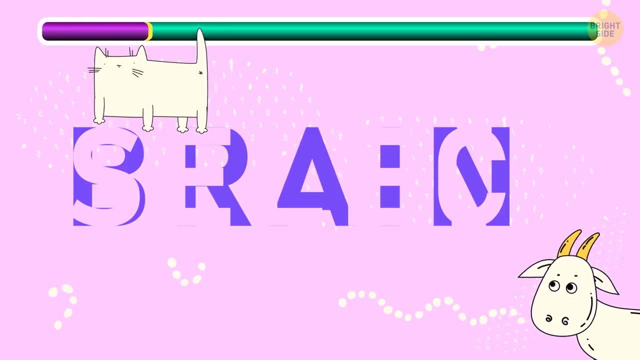 Then you can see it's July. How about this one? It's the word run hiding in the back. Another one for you. Hope you found the gold. Here comes a tricky one. It takes some brain power to see its brain. 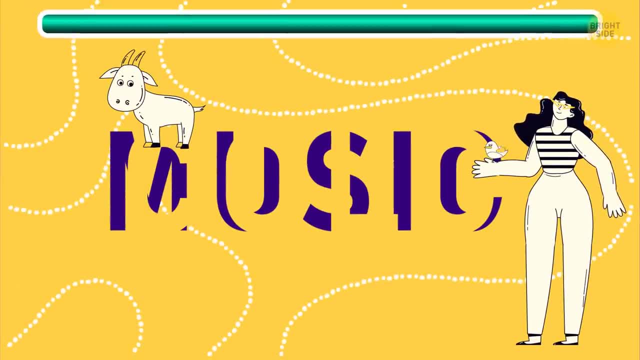 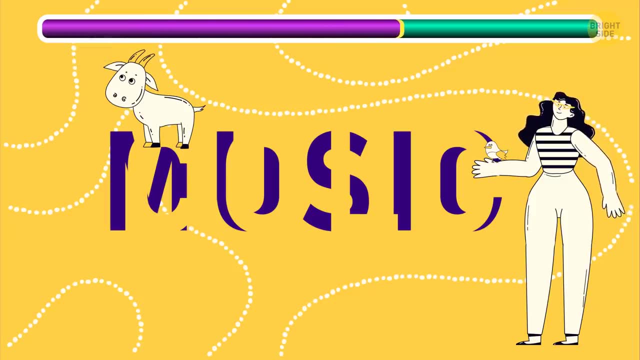 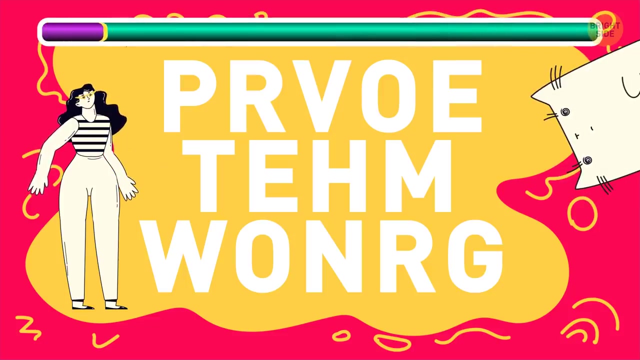 Another one in this category. It's only getting more complicated. If you read the word music between the lines, you must be a genius. Now let's see if you can decipher these secret messages. I give you 10 seconds for this one. 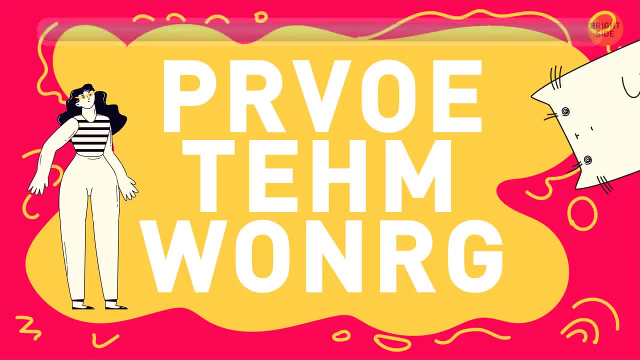 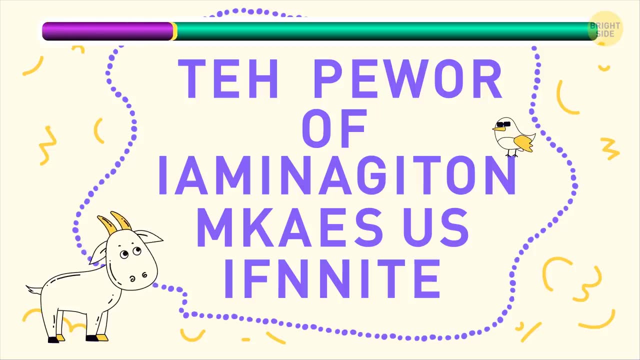 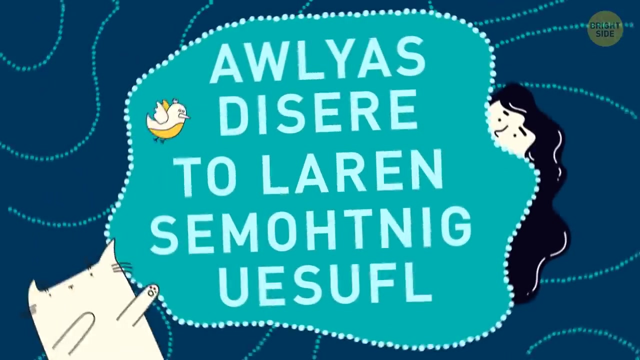 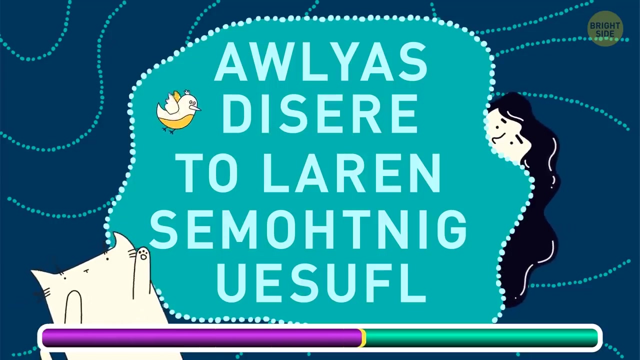 Well, if someone says it's just a bunch of letters without meaning, you can easily prove them wrong. What do you see here? The power of imagination makes us infinite. Couldn't agree more. Here's another one. I hope you always desire to learn something useful. 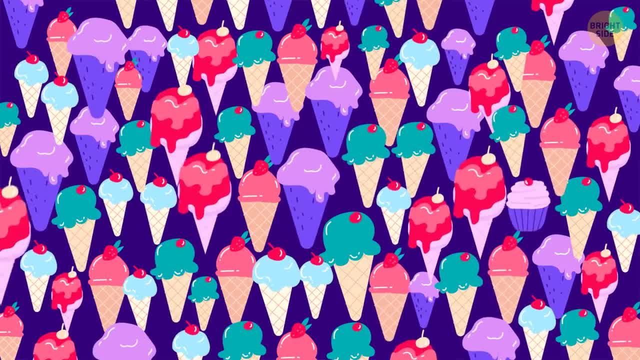 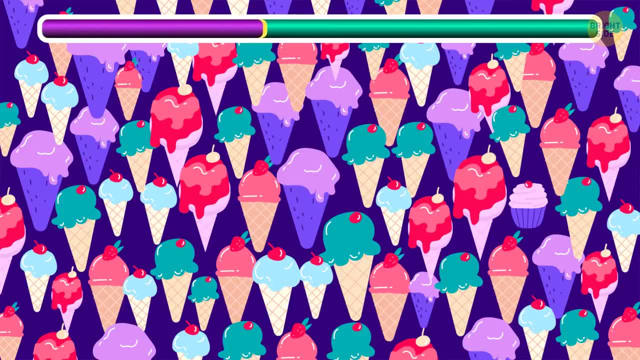 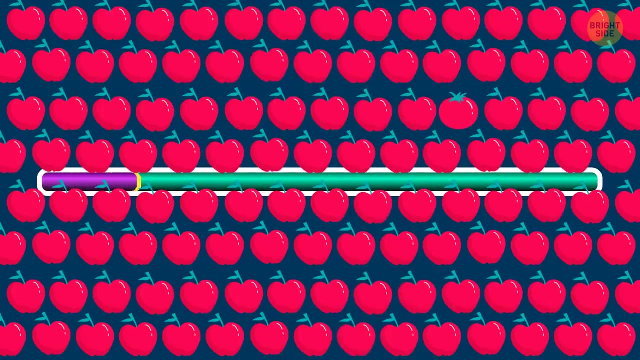 You deserve some dessert for all that mental activity. Here's just one cupcake among all those ice cream cones. Try to find it. There it is Yum. Get a tomato to go. I can only see a bunch of apples, But maybe you'll be luckier here. 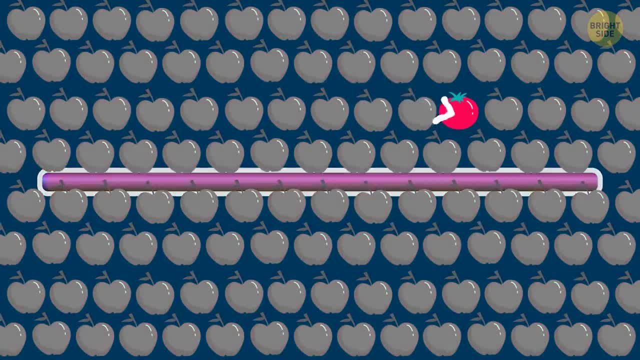 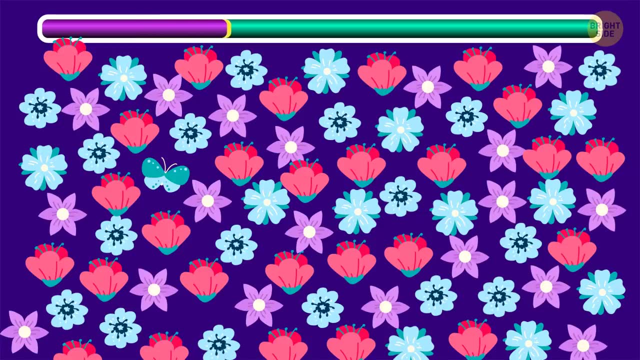 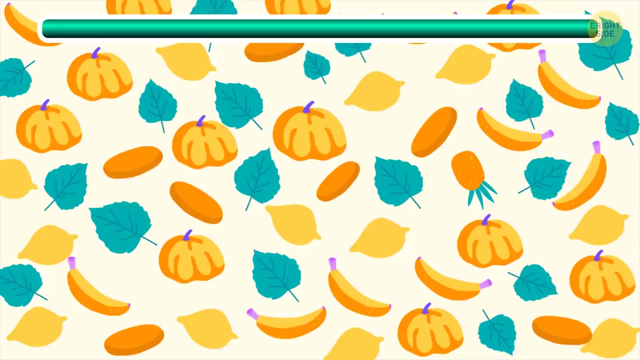 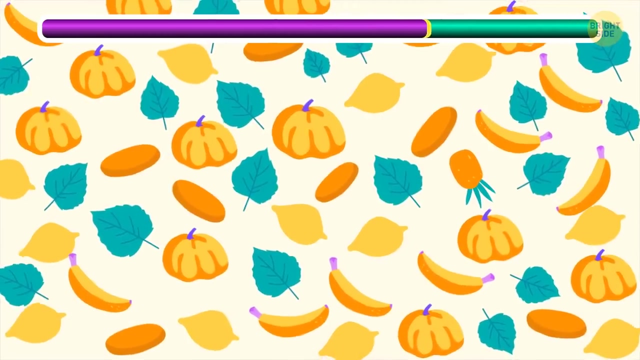 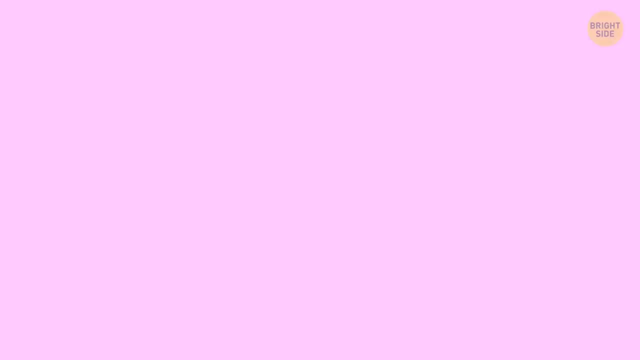 Found it. There's a butterfly hiding somewhere among those flowers. Do you see it? Fantastic, It's right there. Can you find the one and only pineapple in this image? Great job, One of these colorful leaves is in fact, a mushroom. 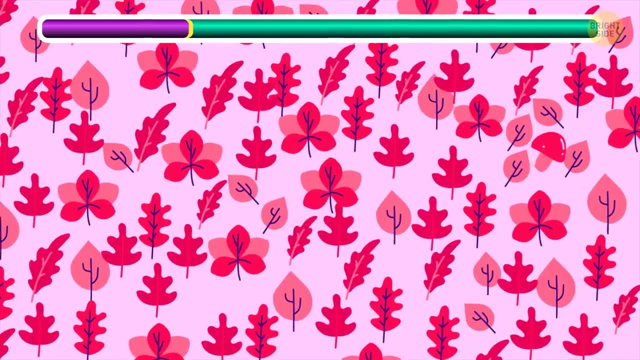 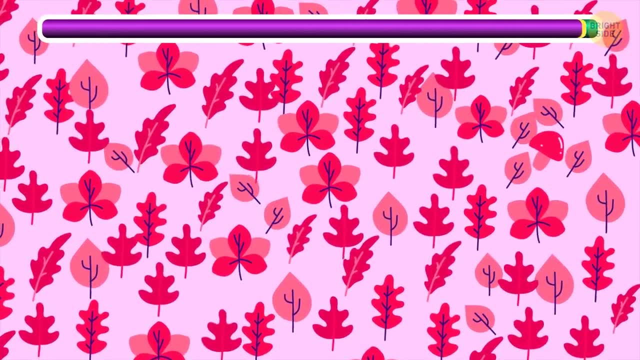 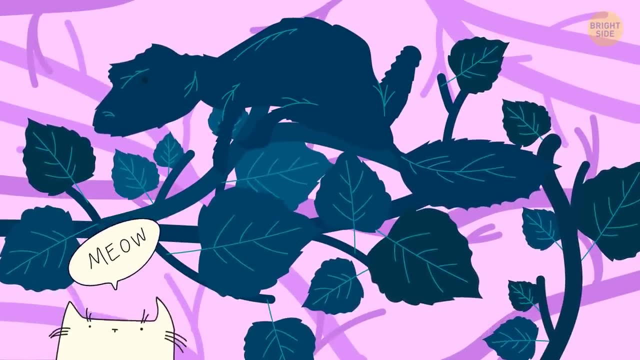 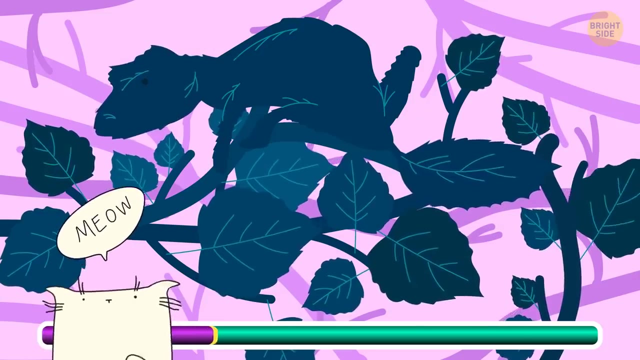 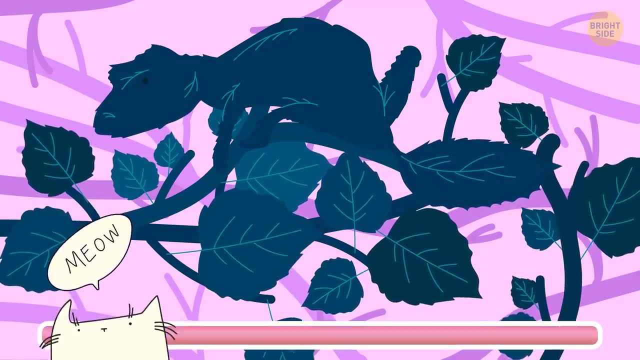 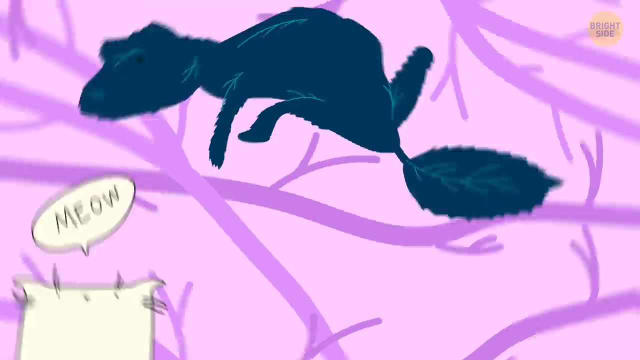 Can you spot it? Well done. How about a safari to give your eyes another test? Do you see anyone hiding in these leaves? Yep, It's a chameleon, And those guys know how to blend with the surroundings. There must be a groundhog hiding somewhere in the rocks. 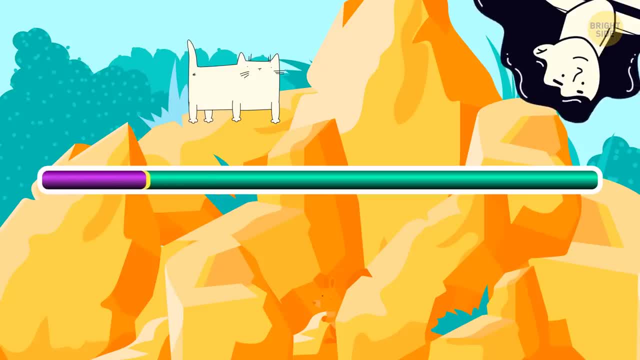 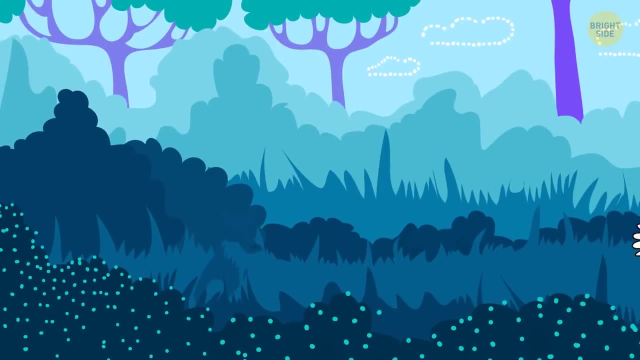 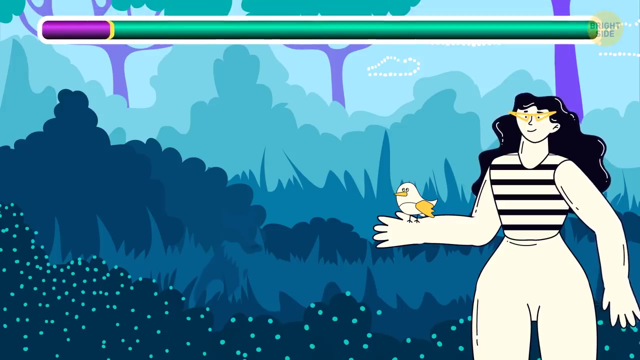 Find it in 10 seconds. Find the best spot And let's go. Wow, that was neat. One coyote won't do you much harm, But if it brings some friends, better make sure this area is coyote-free. Start looking for a different picnic. 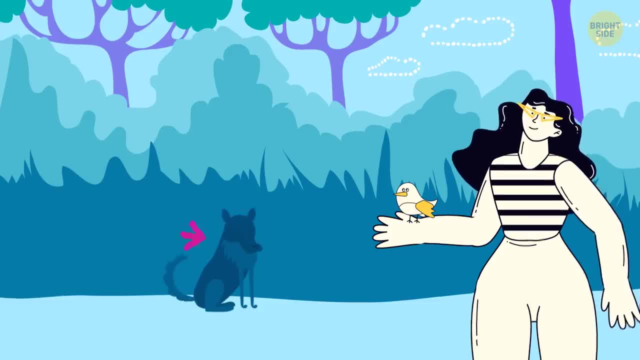 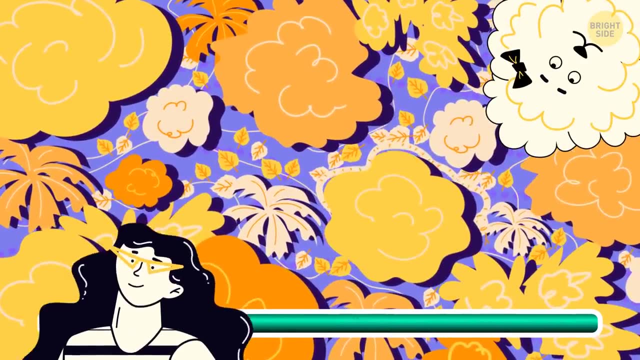 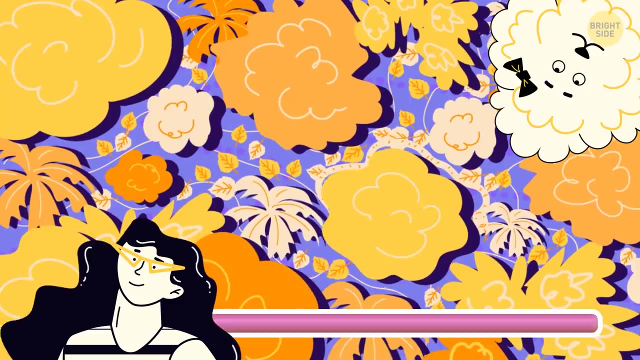 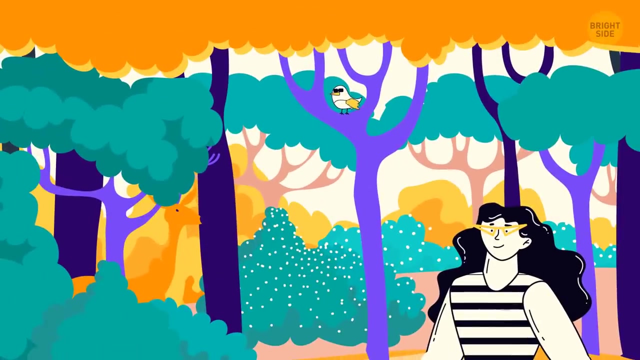 Start looking for a different picnic spot. one of those guys is right here. watch where you step. I hear there are snakes on the ground. found one. better be careful. I don't see anyone roaming in this territory. let's see if you have sharper eyes. what a beautiful gazelle did you manage to find. 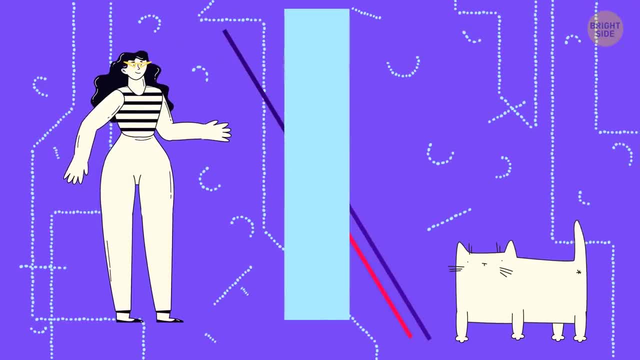 it. the next illusion was created back in 1860. it shows how your brain perceives depth and shapes. so do you think the black line lines up with the blue one? if you answered yes, you're wrong. in fact, the black line stems from the red line. 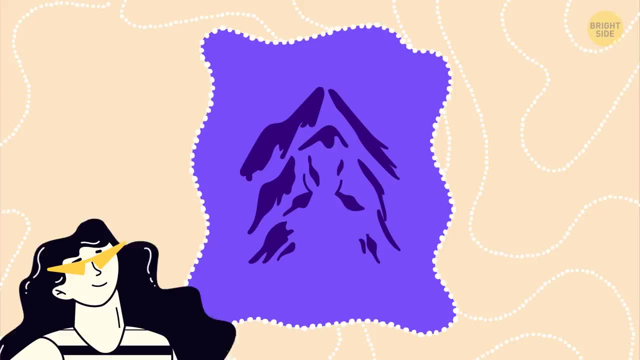 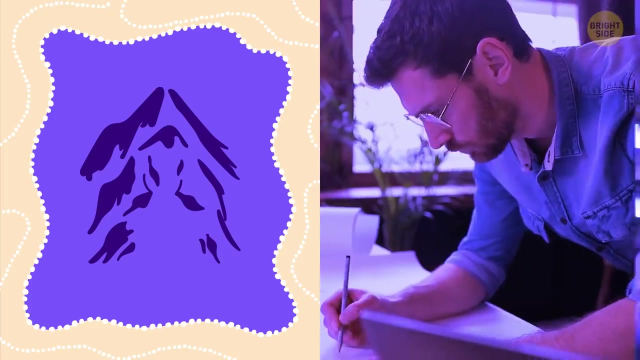 now take a look at these illusions and remember what you see. first, it can tell a lot about your personality. if it looks like a mountain to you, you're a down-to-earth person. you're persistent, reliable and like to plan things. overcoming obstacles makes you feel really happy. you appreciate stability and don't like to take risks. 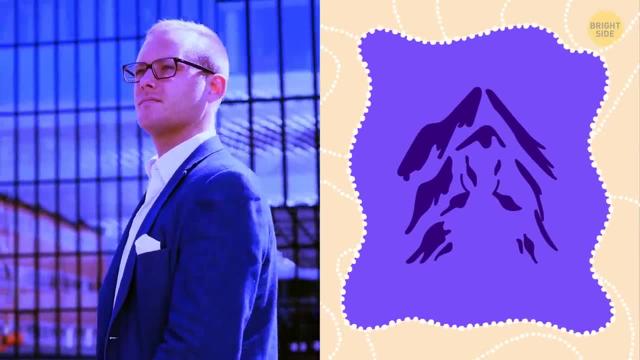 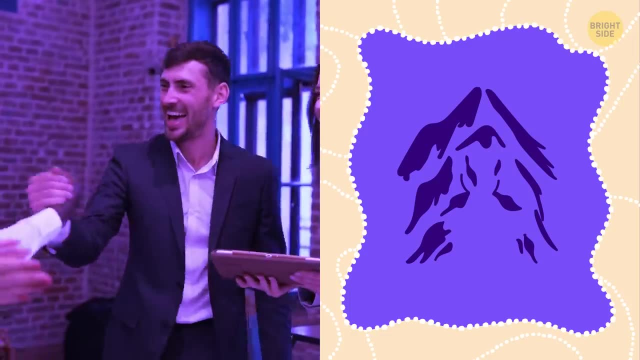 if you saw the upside-down wolf first. you're a natural leader. you keep your emotions under control, even in the most stressful situations. others admire and respect you for that. remember it's okay to ask for help sometimes if you need it. how about this one? if you're not sure what you're looking for, you can look for a. 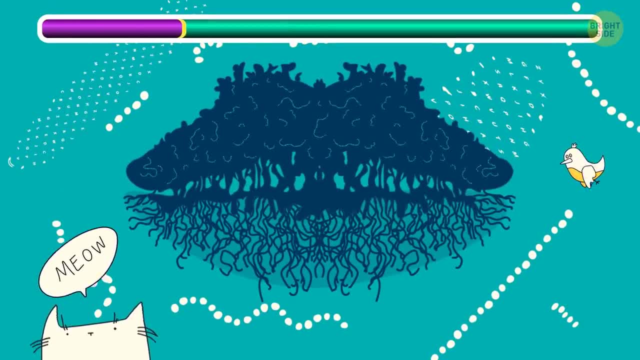 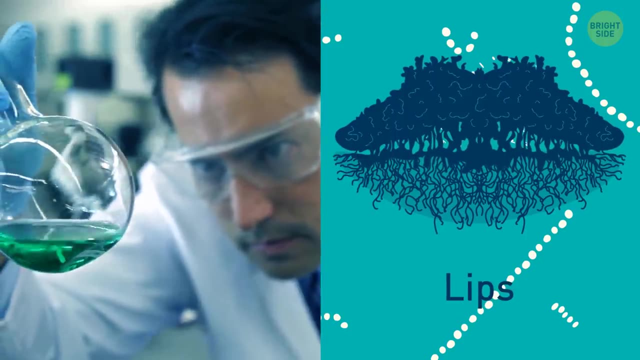 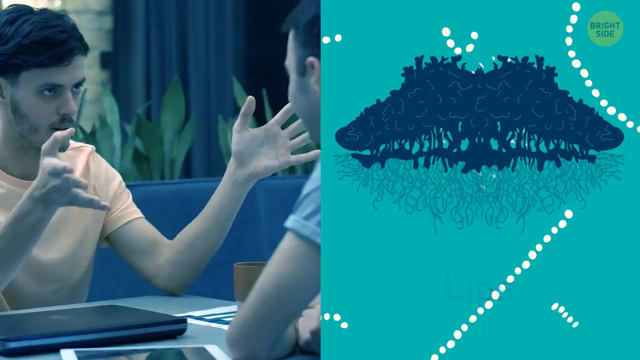 chance to find out what you're looking for if lips caught your eye first. you're realistic and always take things the way they are. you don't look for hidden meaning in what happens to you and what others say to you. it helps you get along with people well if you notice the trees. 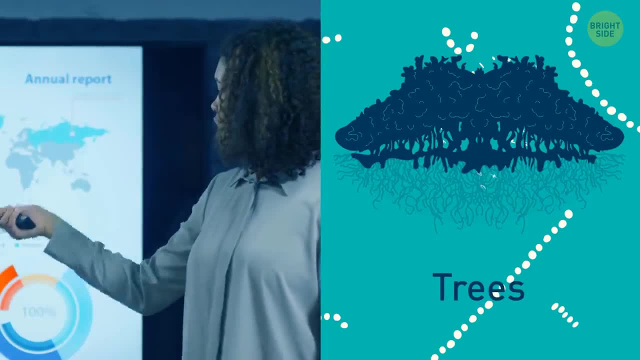 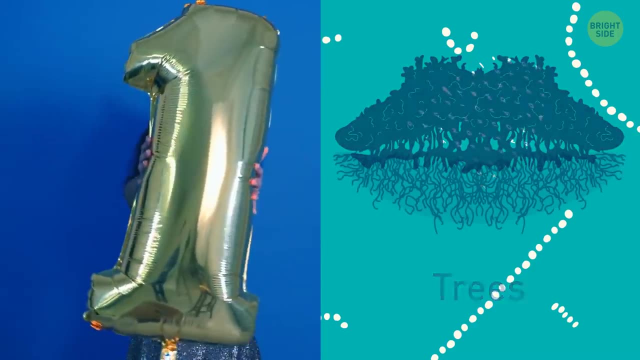 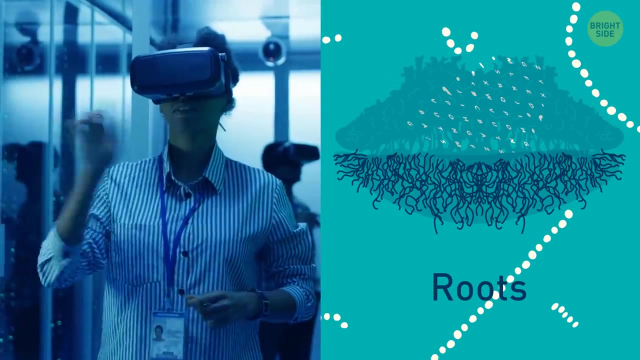 first. you're an ambitious person and a perfectionist to the core. you're never happy with just okay and will always strive to be number one and make yourself and others happy. in the case, the first thing you saw was the roots. you're an extremely progressive person. you love trying all the new technology. 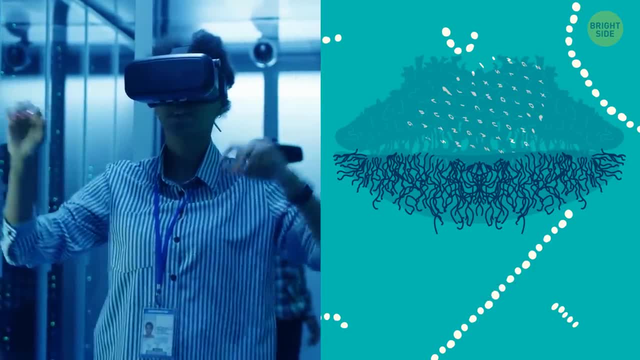 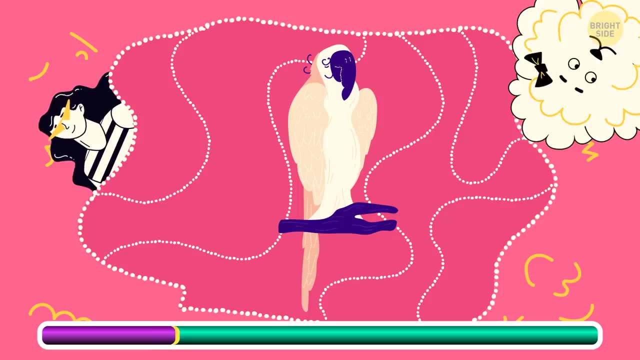 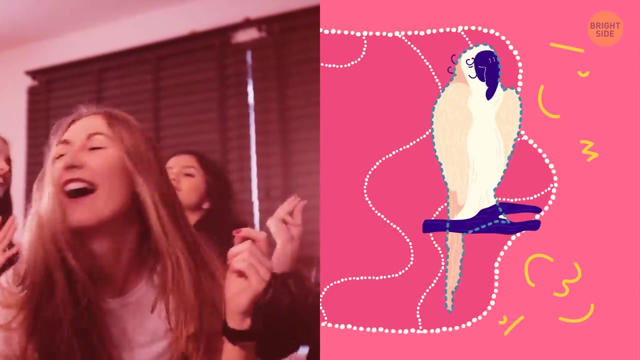 and styles. you never settle and always try to make your life better and more exciting. here comes the next one. if it looks like a parrot to you, you're the soul of any party. you like to be the center of attention. wear something bright, talk loudly and laugh your heart out. you have plenty of 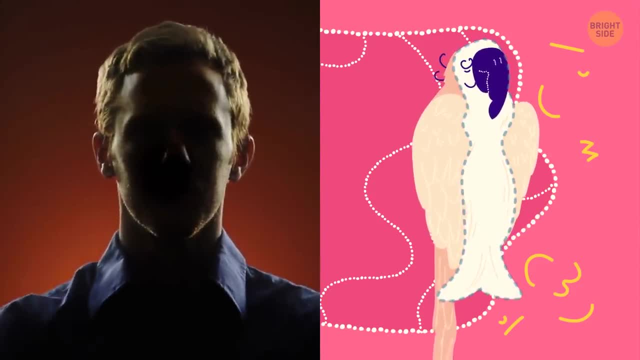 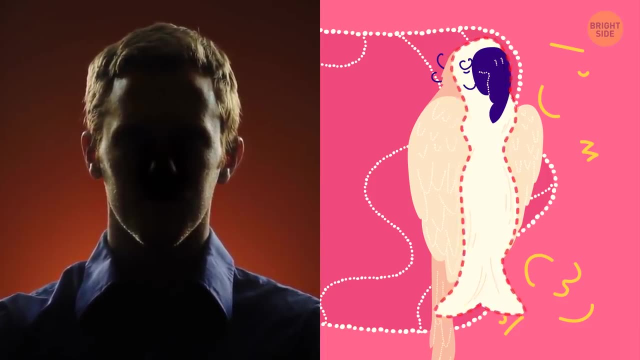 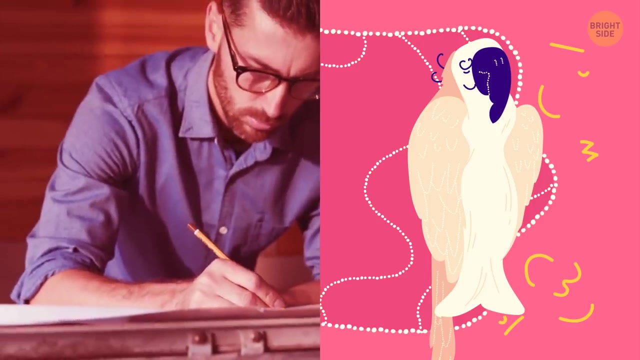 friends who love that about you. if you see a girl in a beautiful long dress, you must be the mysterious artsy type. you prefer to observe others being active and loud and get inspiration for your work. you notice little details and remember them to later put them on your canvas or paper. you have 10 seconds to decide what you see in this illusion here. 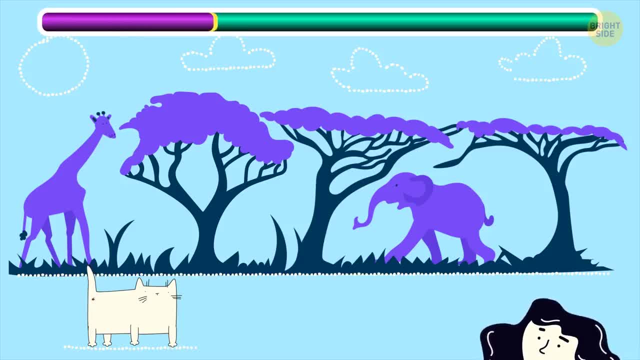 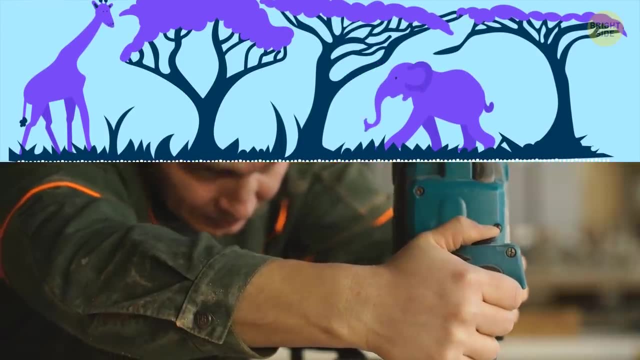 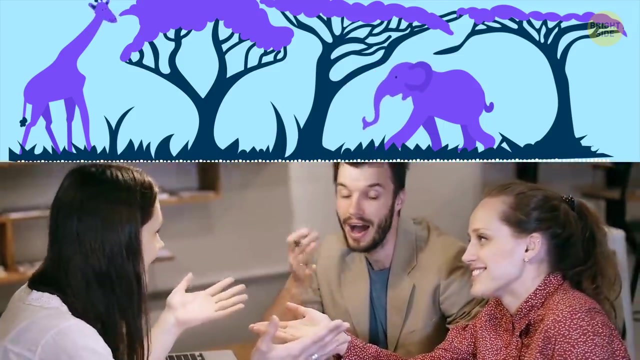 if it's clearly an image of an elephant and a giraffe. you're a reliable and hard-working person. you feel responsible for yourself and your work and don't like to let others down. people appreciate you for that and share their secrets with you. if you saw some. 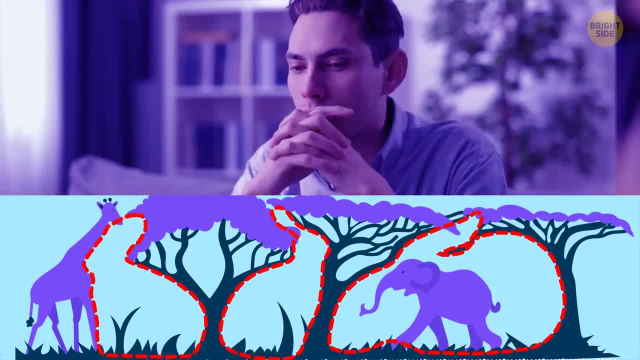 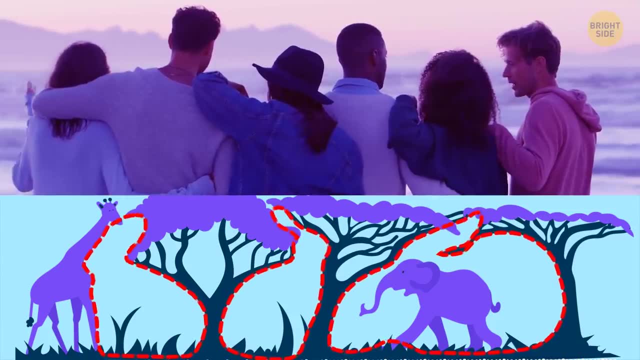 rabbits between the trees. you're not as simple as you might seem. you always think before you say or do something. you have a strategy for every life situation. it's important to you to be accepted and loved by others, so you do a lot to please them. new illusion same. 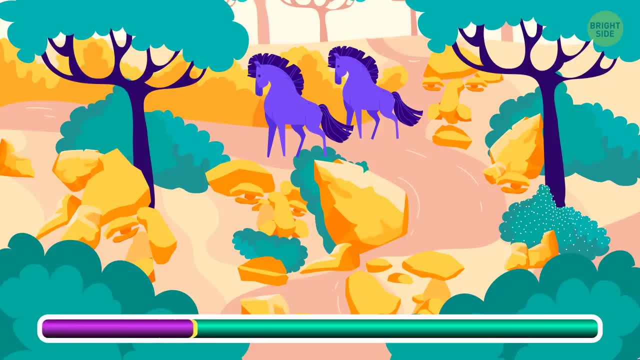 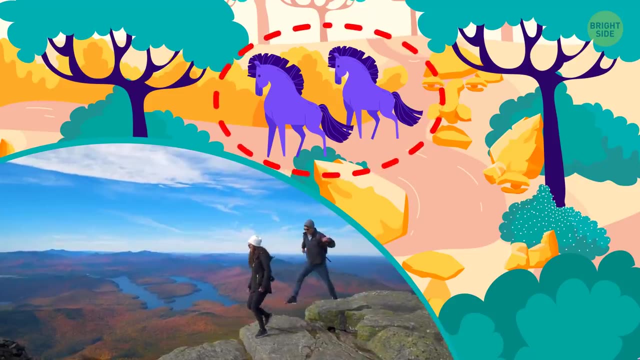 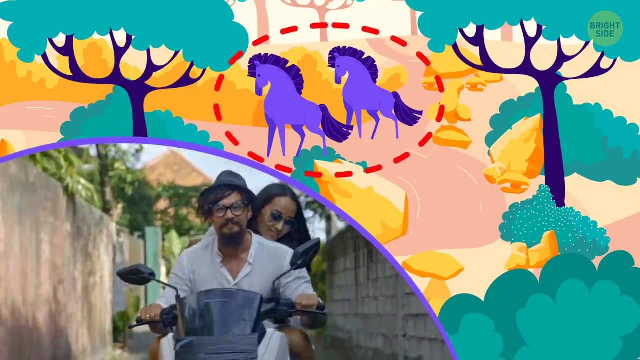 task if you see just two horses crossing a waterfall. you're an adventurous person. when someone offers trying something new or going to a new place, you're always up for it. you realize you might not like it in the end, but you'd rather try it and be sad than regret not going. 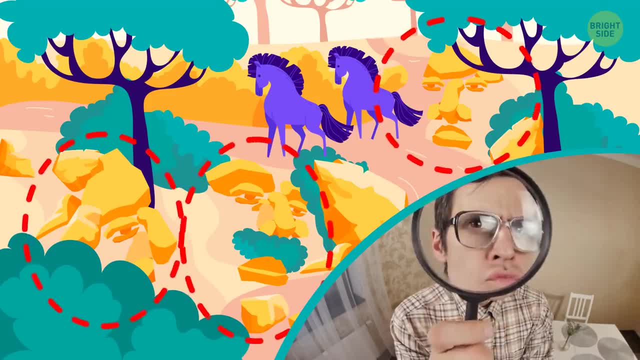 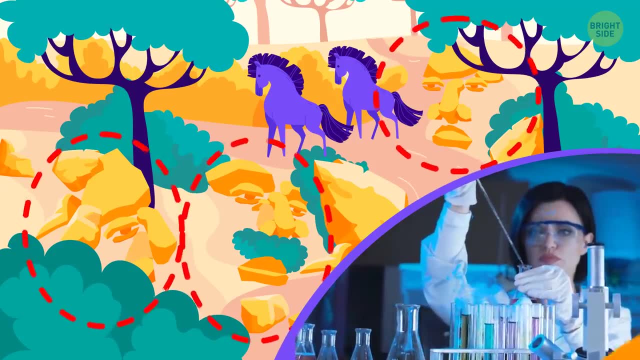 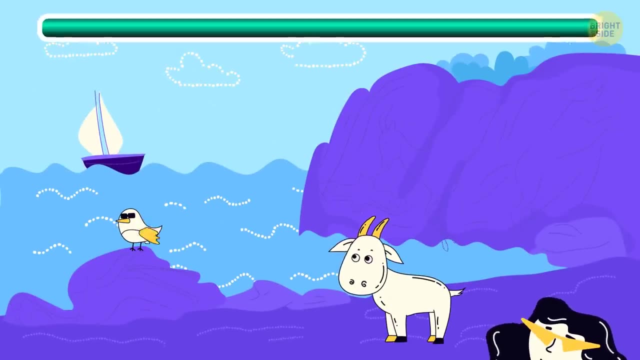 in case you noticed several faces first, you always see the big picture and can find the right decision quickly. you know what you want and how to get there, and never reconsider your own choices. these qualities will take you far in your career, moving on. what a beautiful landscape, but is it hiding something? 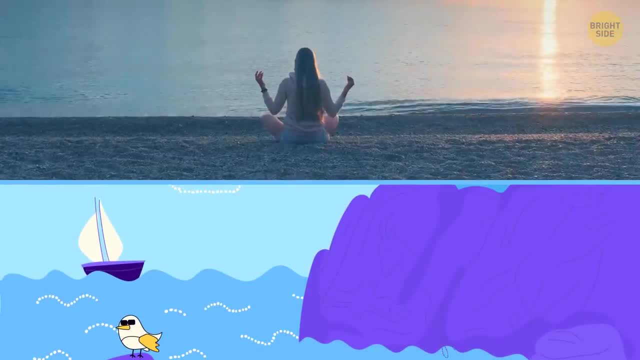 if all you see here is some sea and rocks. you're a calm and balanced person. sometimes you're in a bad mood, but you always look on the bright side of life and move on. you're a calm and balanced person. sometimes you're in a bad mood, but you always look on the 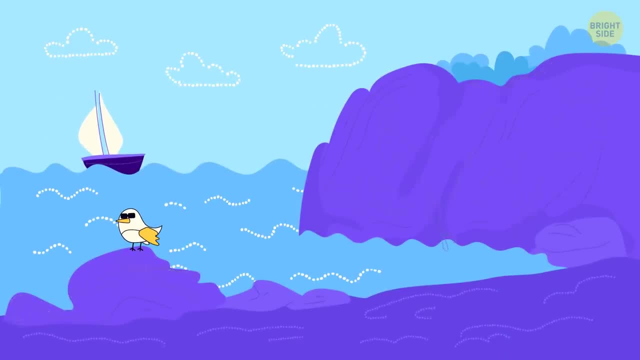 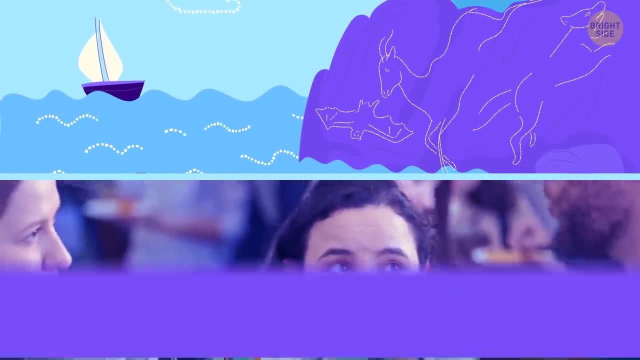 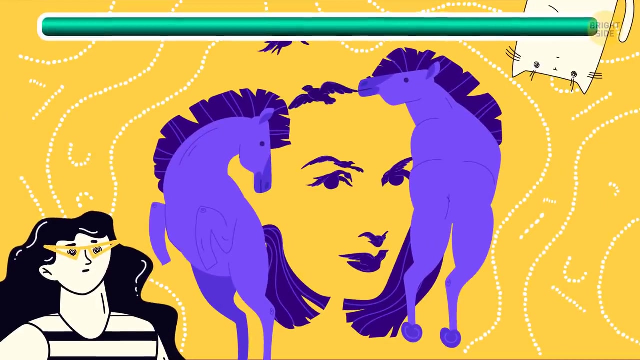 bright side of life and move on. when you get lucky. you're in a bad mood, fortunately, because this style is veryNote on the rocks. you have a great eye for detail. you always listen to both parties in a conflict before taking science. you like doing research and drawing logical conclusions. all right. 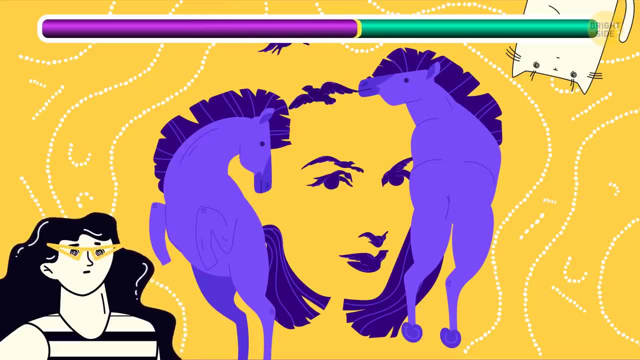 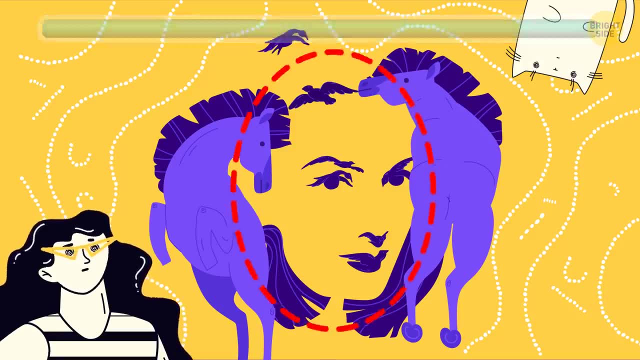 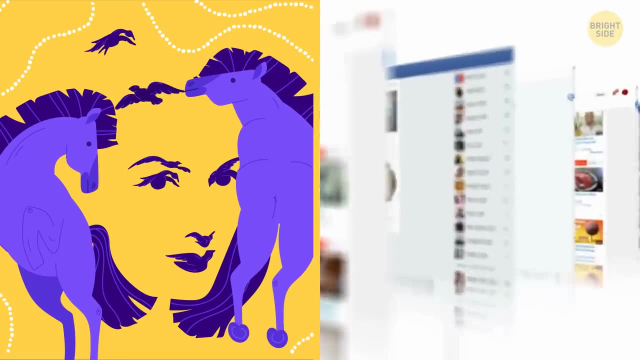 what does this one say to you? in case you're positive, it's a portrait of humans. a young girl, you're an extrovert and can't survive a day without people. you're active on social media and enjoy going to social events, where you can make even more friends if you see some horses. 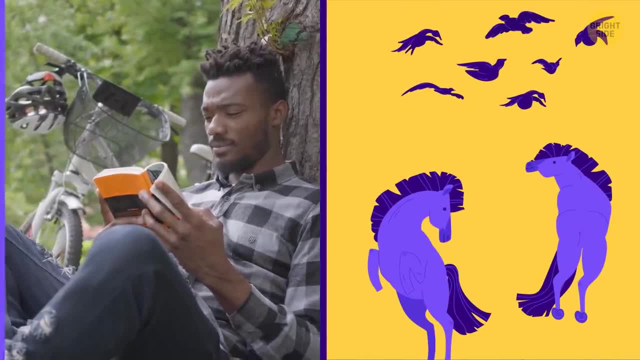 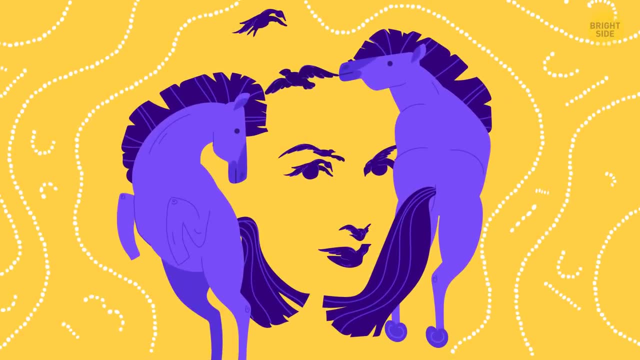 and birds. you're more of an introvert. you love being alone outside. you have some great friends, but you appreciate your personal space, those who see the face and the horses at once. you've got the best of both worlds. you feel comfortable at a party with a few hundred new people around. 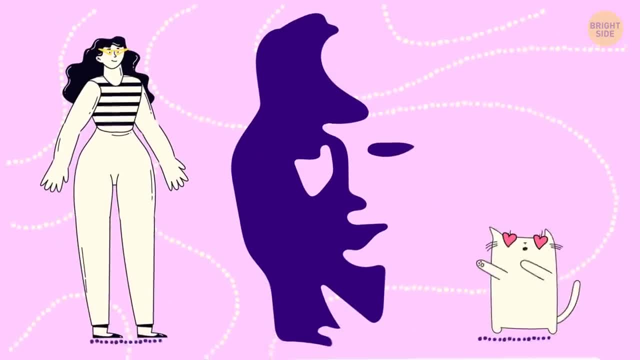 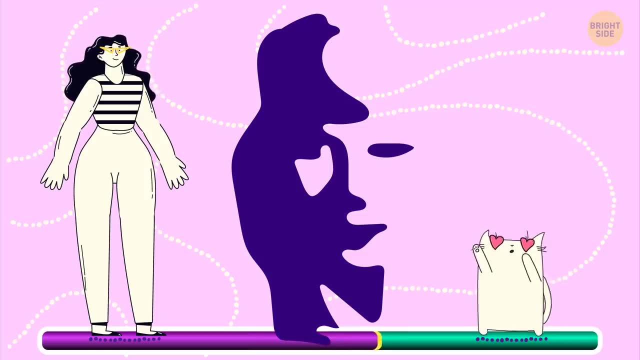 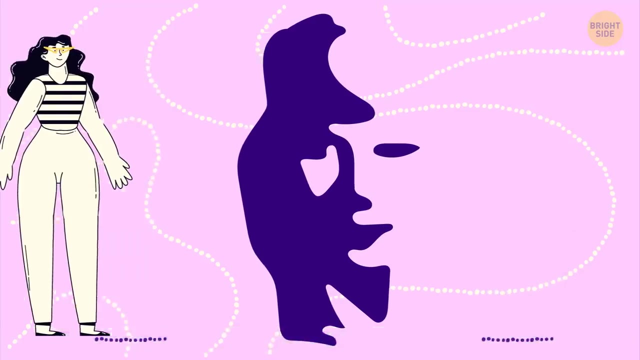 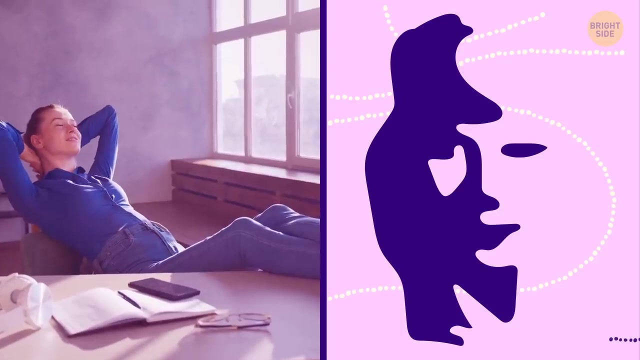 and alone reading a book. what can you say about this illusion? those who see a face of a woman. you're realistic and pretty content with your life. you don't expect too much from others and are ready to stand your ground if you have to. if you see a saxophone player, you often prefer your. 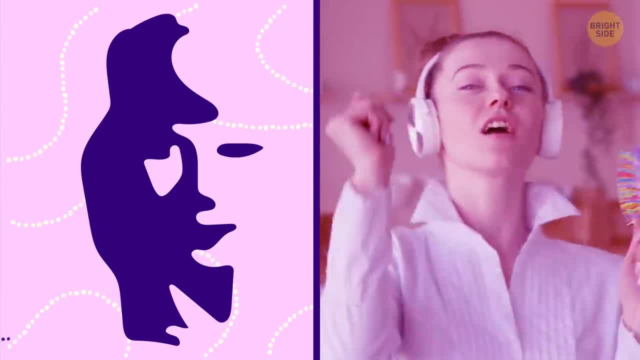 imagination to your personality. that's why you'll be ready to stand your ground if you have to. you often prefer your imagination to your personality. that's why you'll be ready to stand your ground if you have to. world to the real one In your dreams, you have turned your favorite hobby into a